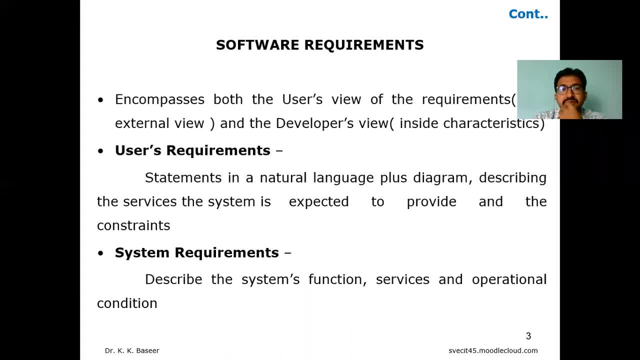 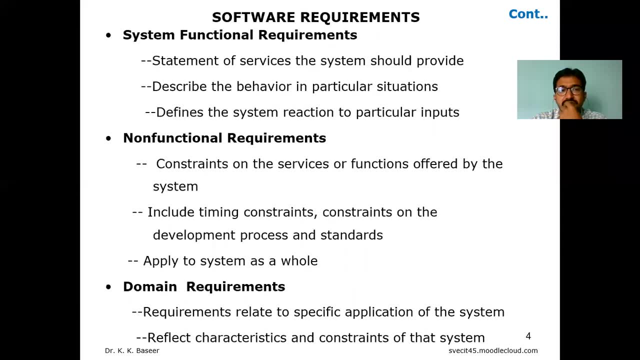 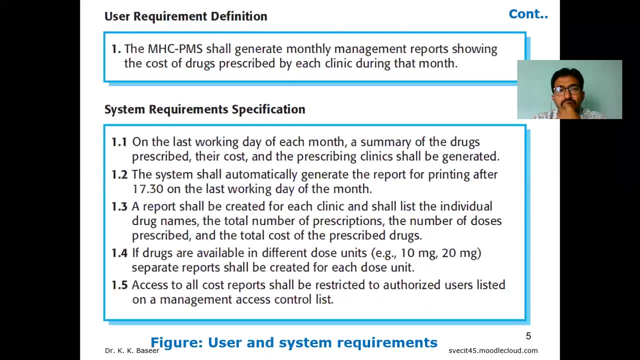 also called as requirement. Also we have seen the different types of software requirements Under that, the user requirements, system requirements. Again, in the system requirements there are some sort of categories like system functional requirements, system non-functional requirements, the domain requirements, all sort of stuff. with small examples By taking MHC, PMS example: 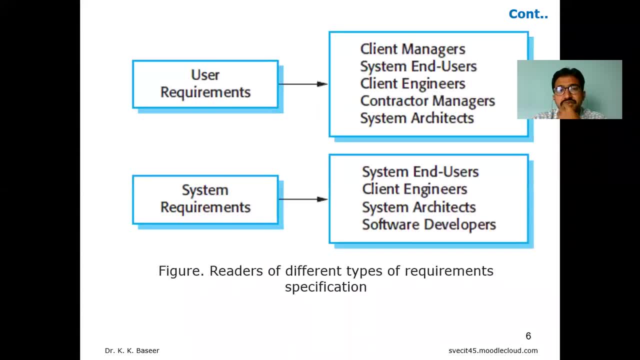 we have seen over there And we have also seen what the different roles or the persons involved in the system are like. So we have some categories like system functional requirements is a requirement as well as in the system requirement. now let me go for. 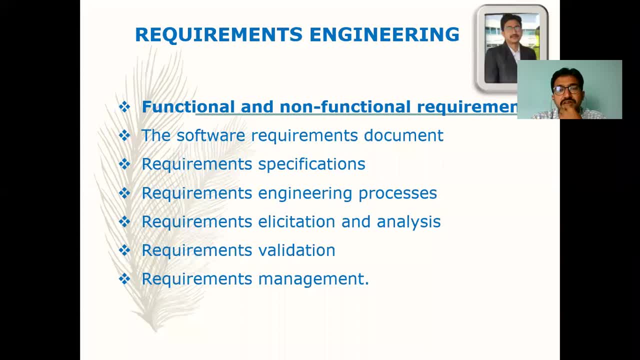 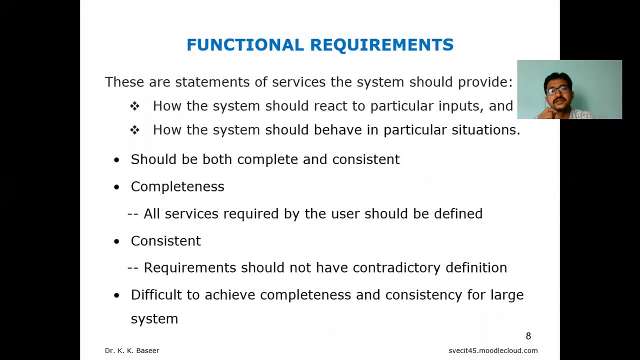 today. the first topic: functional and non-functional requirement. see in depth of this one, let me discuss little bit more detail about functional requirements as well as non-functional requirements as a part of this. let me start with first one: functional requirements. the functional requirement: as I said you in the previous class that if you are defining that requirement in 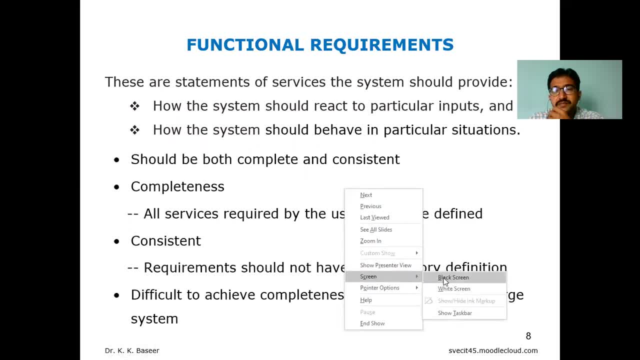 the form of a statements, for example. the statements can be the statements. these are statements of services. these services is the first services, how the system should react to a particular input. as we talk about function, normally function means what to do to complete a particular task- is called as functional- functional in the sense. 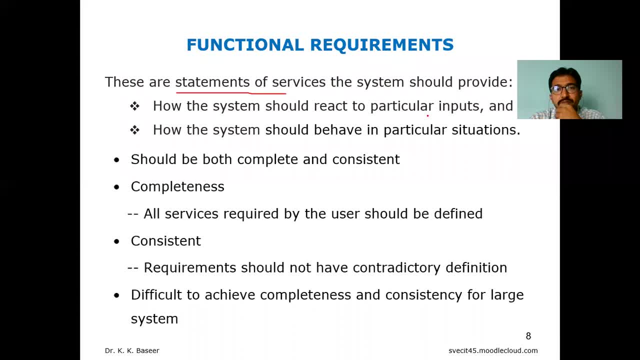 for a given input, whether the desired output is. comes or not, the middle, the process, how we are going to be make man play, make managing and operating with that inputs to get the desired output is called as the function in between the input and output. this functional requirement relax now how the system 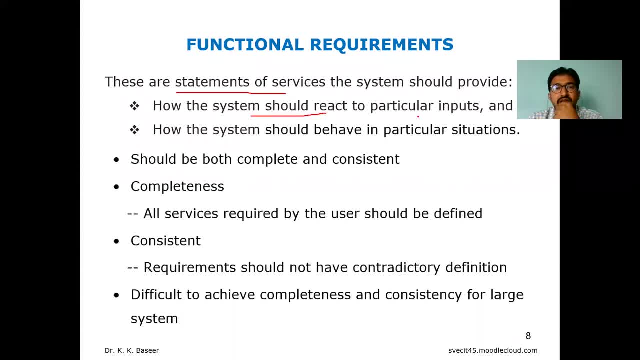 will react for a given set of inputs. how it will be reacted when I wrongly press any button. how the system will react when the wrongly I can give the input. how the system will react when I giving the the input. how the system will react when I giving the. 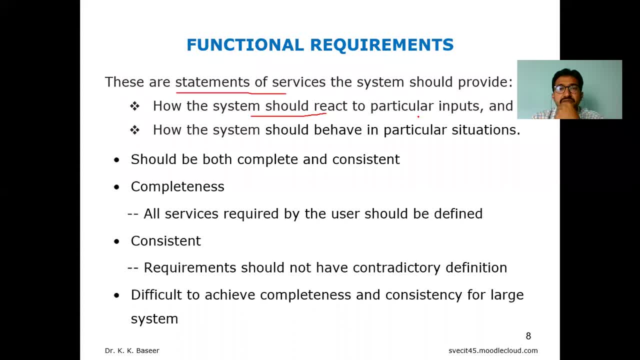 exact or the true input, how the system will react when I am giving by mistake. how the system will react now the second service or the second statement has to observe is how the system should behave in particular situations. so these are the two points, or two statements, where it is going to be concentrating in the 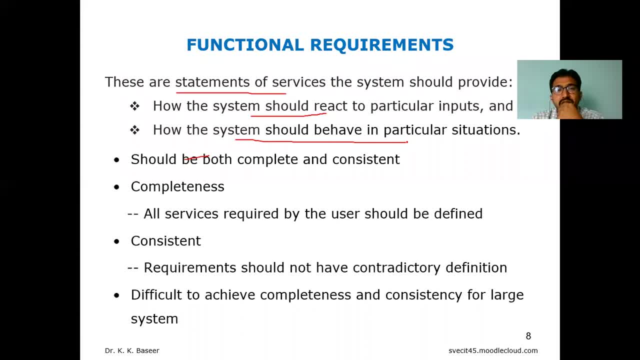 functional requirement, how it will react for a given input, how it behave in a particular situation. so it should be both complete and consistent. as we discussed previously, completeness is nothing but by the user should be defined whatever the user has asking for you to complete a particular task, if it. 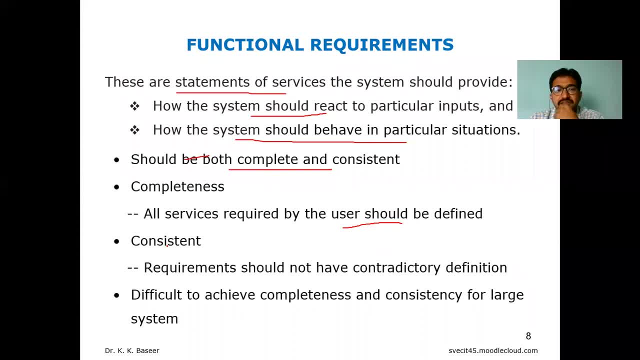 will fulfill, then it is called as completeness. consistence means should not have any contradictory means. there is no partially completed, partially satisfied. it should be very transparent. there is no compromising in the requirement, compromising in the fulfill of particular tasks. so there is no contradictory definition. if it is not there, if there is no ambiguity in the requirement, 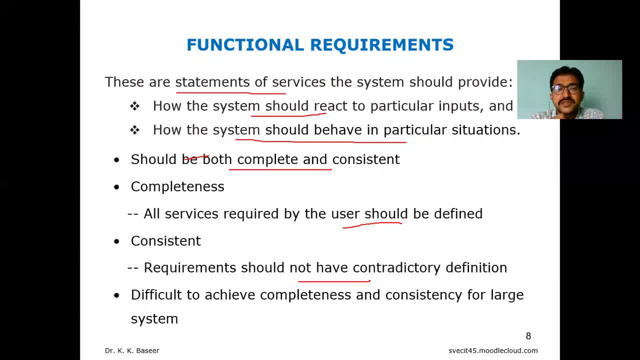 satisfaction, then it is called as consistence. completeness means all the services, whatever the thing the user is asking to the developer or to the stakeholder. all should be has to satisfy. then it is called as completeness. so both should be to achieve this one, completeness and consistence to achieve. 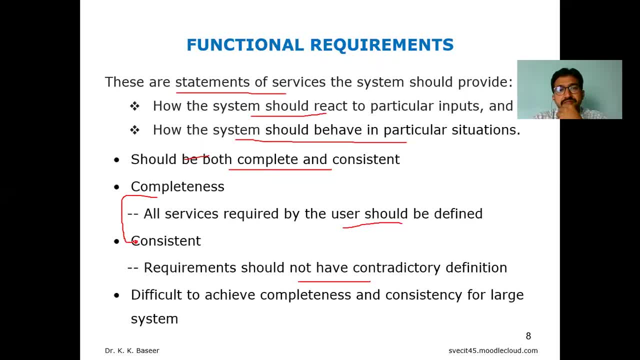 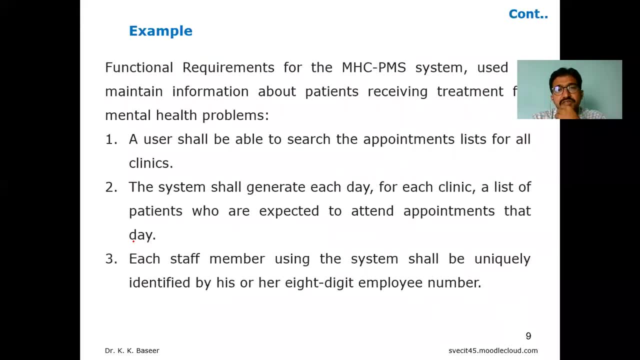 this one. it is a very difficult task for lot system, right? so in simple terms, it is a very difficult task for lot system, right? so in simple, the functional requirements can be say as how your system behave for a given input, how your system will react for a given 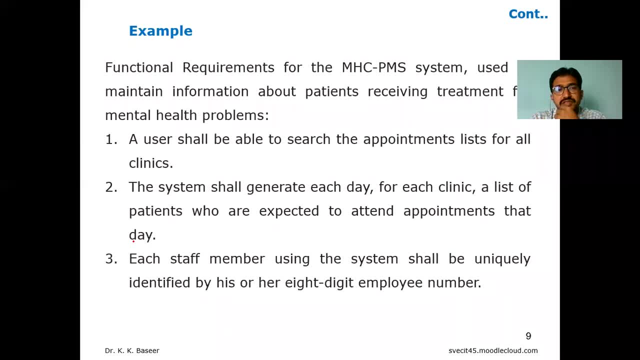 input and how your system is here for a particular situation. take an example, as already we have considered this example, that is, the MHC PMS system. this MHC PMS system we are going to consider over here for functional requirements. now let me see. whatever the functional requirements, 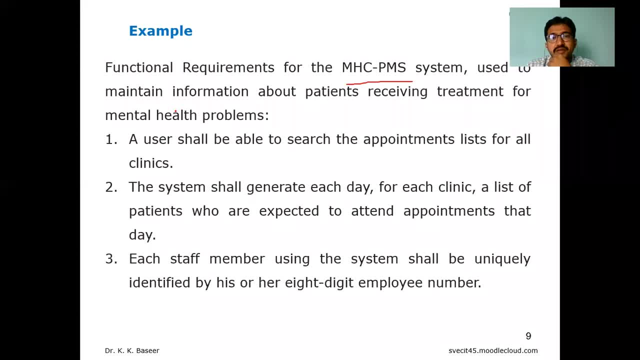 for this project. the name of the project here is mhc pms. now to maintain this one about patients receiving treatments for mental health problems, the first functional requirement is: a user shall be able to search the appointments list for the clinics means if your system is providing. 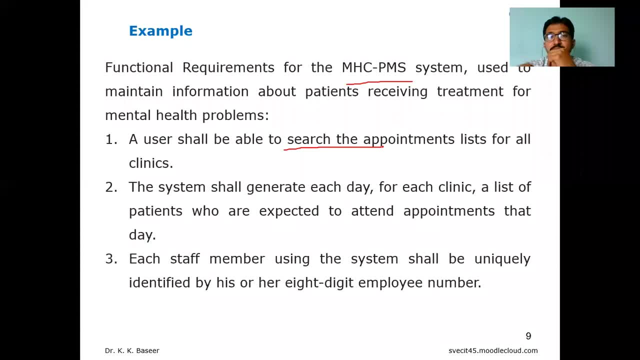 the different services. you had to give the input a search button or a search field where it search for the appointments of the different clinics. your system has provided different clinics of that. so different clinic means based on the uh, these symptoms of disease, they can search for the different clinics over there. the second part is the system shall generate each day, each day, for 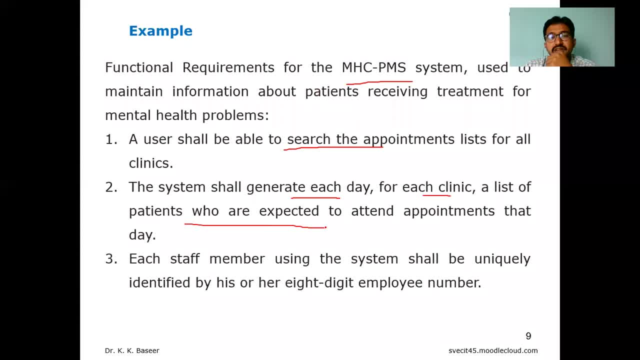 each clinic a list of patients who are expected to attend the appointments that day. the third functional requirement is the staff member using the system shall uniquely identify these are our eight visits. employee id or employ number: eight digit employee number, in the sense, like you have a 10 number. 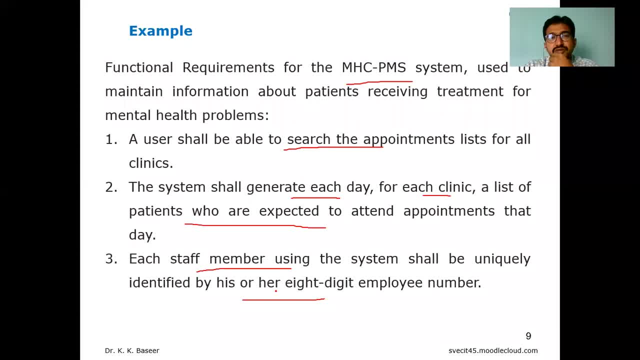 digit of row number, here also at eight digit number. so these are the some of the functionalities that can be provided in mhc pms system. that is a project, so searching is one, generating of report is another, and giving a unique id for each staff number having a eight digit number is another. 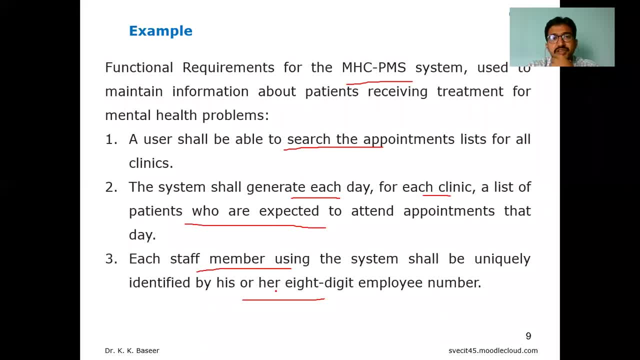 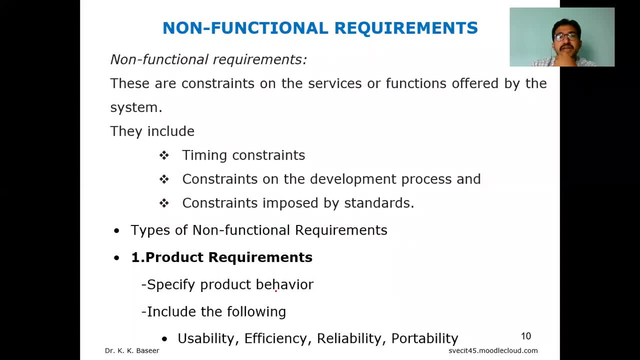 functionality of that particular project. so, in the same fashion, you please apply for your respective project, which you have done for week one, apply for that as well. coming to the second part of the concept is nfr, where nfr stands for non-functional requirement. now, here, when you talk about non-functional requirement, it deals with 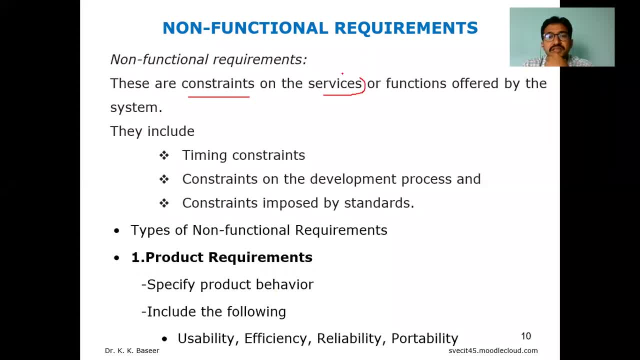 constraints in law, in the functional requirement will deals with the functionalities, means, services that are going to providing by a particular project or a particular system. now, under which conditions, under which constraints it will be satisfied this service, it will satisfy. for that, that will talk in nfr. so simply, nfr deals. 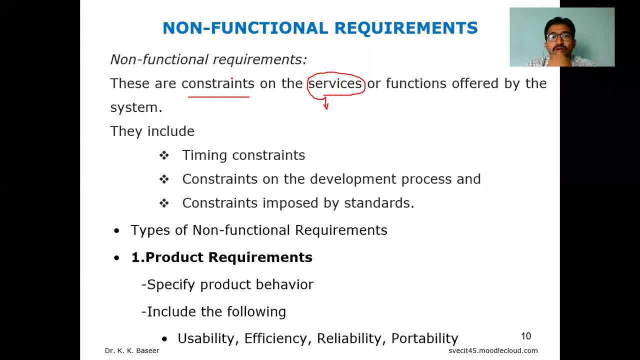 with the constraints or conditions where it applicable. now, what are the different types of constraints or conditions it is going to be concentrating is? the first is time, time constraints under what timings it has to be completed. that particular request or particular service? maybe, if your request for a transaction, for example, or when you are searching for mhc, uh, the system itself. 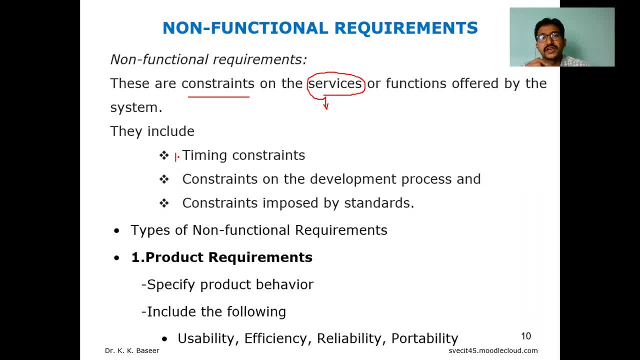 ms system, you are searching for an appointment for a particular clinic. now, when you are entering a query, how in within how much time the response has to come? there is a time constraint: within the three seconds or two seconds or two milliseconds or 10 milliseconds? how much of time it has to? 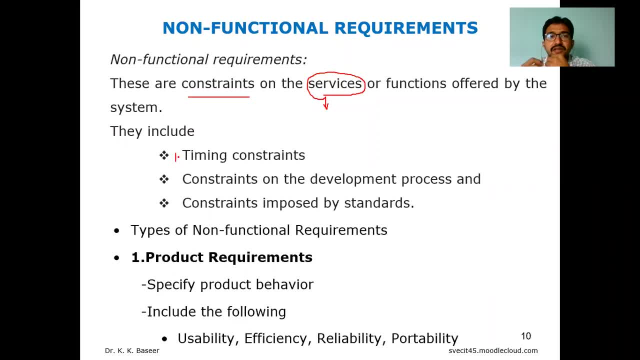 complete that service service. giving a service means giving a fast service. if you are giving for a 10, 10 days of service, it is a waste of the customer will not satisfy. so very fast track. you have to provide the services. the second constraint is the constraint of the development. 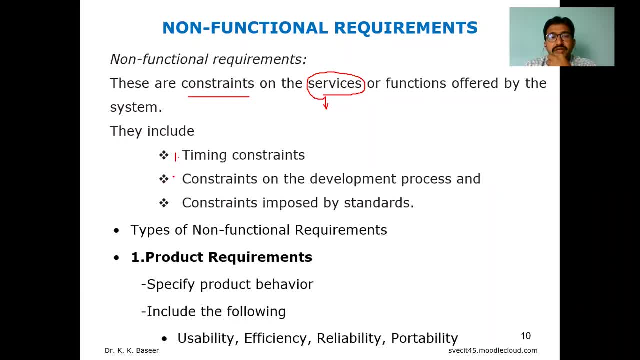 process now, how much of time in fulfill it will complete that. how much of time to complete this? constraints in the development process- now, constraints on the development process is nothing but the minimum requirement: how the configurations of your system should required, how, for what type of system it will be run. all such type of development constraints with the. 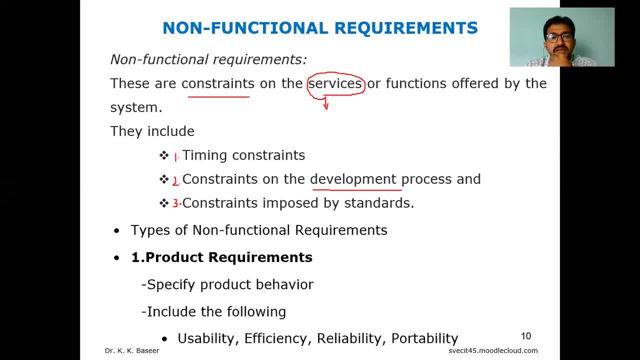 second one. the third constraints is imposed by standards, means it has to follow some standard rules to fulfill that particular thing right. so such type of constraints, when it deals it comes under nfr, where nfr stands for non-functional requirements, now types of nfrs. so already we have discussed in the last class that different types of nfrs we are having under 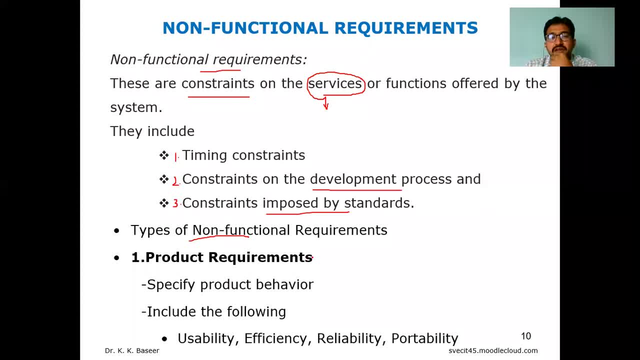 that in a specific way, when it deals with product requirements. product means which can be a logical way or a physical thing, that a product- here the product will be using maybe a software, that product may be a which is integrating in a manufacturing mechanical part or which can our software can be embedded in any electronic devices. that also all cons. 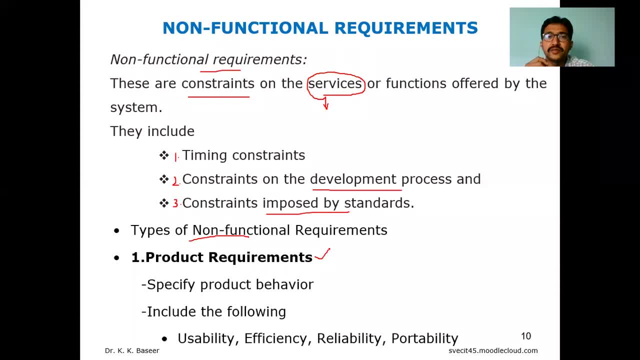 comes under product. so a product may be a software, a product may be which is embedded in a particular electronic device or embedded in a mechanical, or manufacturing physical things. so coming to the first one is the product requirements specify the product behavior, product behavior how you can be measured. the product behavior means you can measure with the. 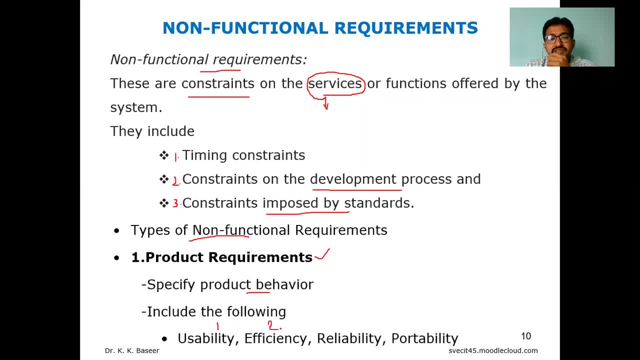 help of the first is usability, the second one, efficiency. third one: reliability. fourth one: portability. coming to the usability now. usability is how good, which type of users and can be used for that one, if you have your own mobile and if you are operating and if you are maintaining that mobile. 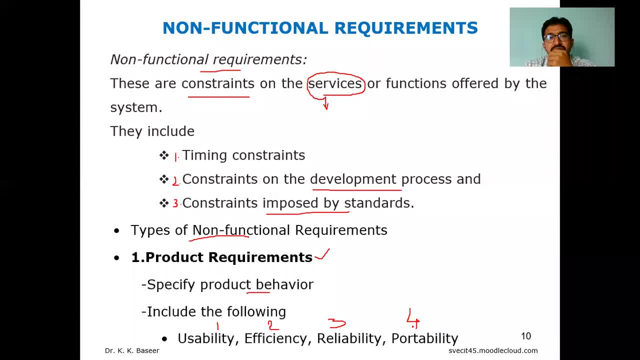 you can. within a long period of time. it can be manageable because whenever the charger is there for charging is over, or any recharges or any maintenance or cleanness of your mobile, everything will take care of. so, based on that, it is a possibility which can give some sort of the 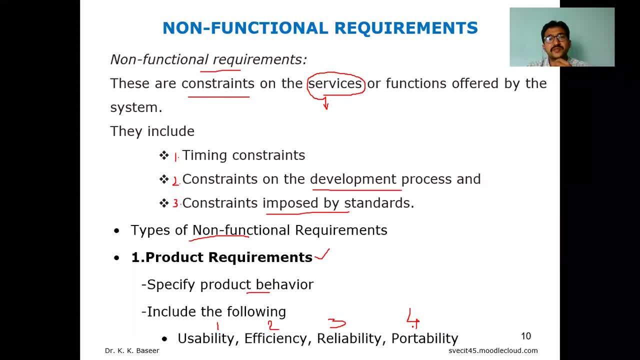 more life long over there. if the same mobile can be used by other parties which is not their own property, then the usage and use of the things is very different. efficiency based on the usability. the efficiency also depends- and reliable, how good, how strong, how many number of days it will be. 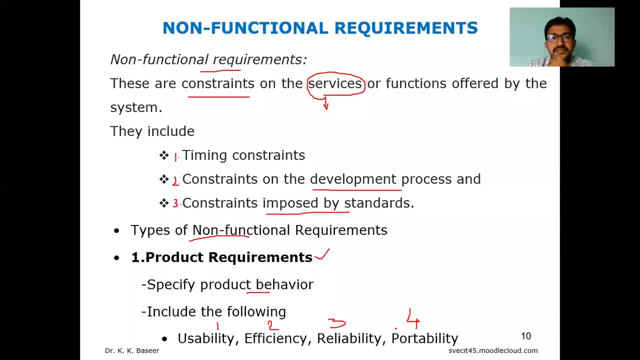 supportable. portable is nothing, but for any type of system java is a portable language means for any type of operating system, maybe mac os or linux or windows. for any type of operating system this is portable. such type of four leds: if you observe the leds: usability, led efficiency. 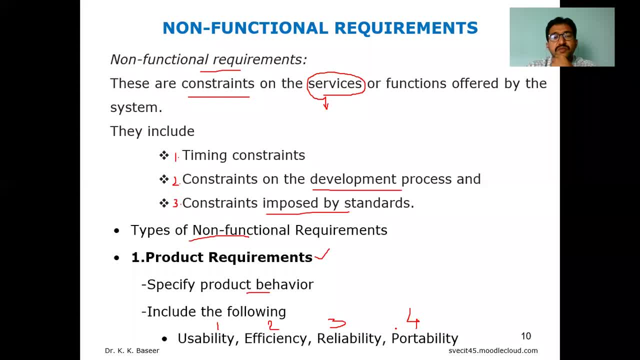 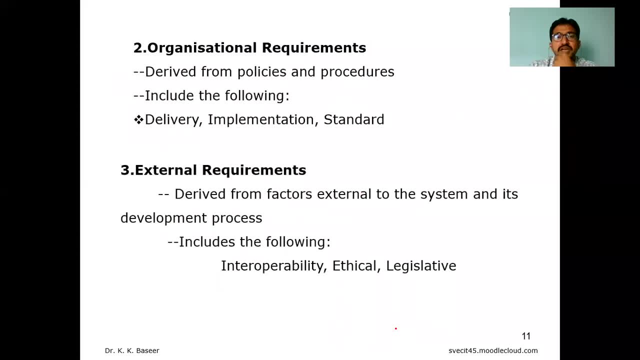 reliability led, portability led. these four things will comes under product requirements: usability, efficiency, reliability, portability. second category of non-function requirement is organizational. organizational requirement is nothing but like companies or like colleges, they derive the policies and procedures. so to fulfill anything, the policies has to define. so what is the policy to join in engineering college? the policies is. 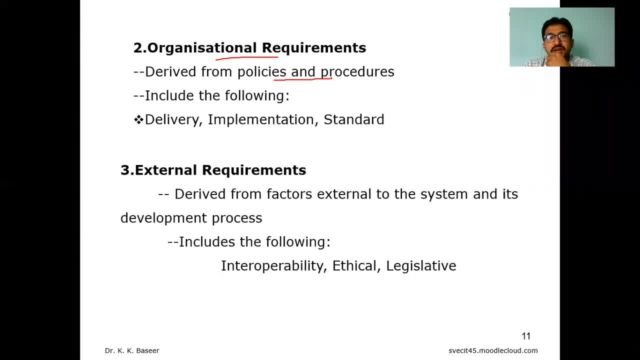 first of all you need to be qualifying less one plus two and or intermediate. after that there is will be an entrance examination and after that, based on the seat, you can allocate it from the quota there will be get and those who are eligible, they can come and join in the convenient quota. 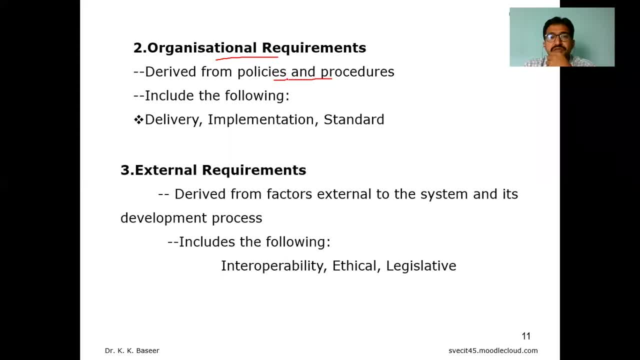 that is the policy and procedure. further, in the same fashion, the processors and policies will be there in the organizational requirement, like in this one, when we have to deliver the project and in which type of things we can be implement this one. what are the standard procedures we need? 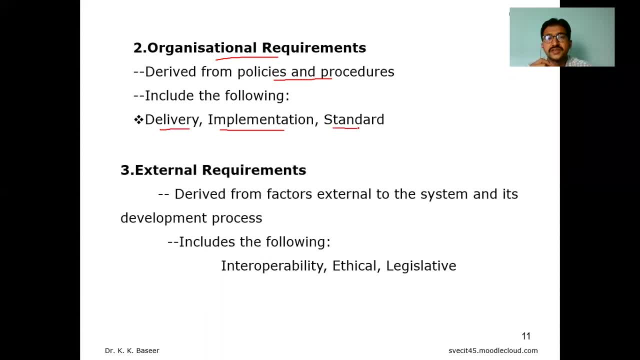 to follow because if you not make some precautions when you are delivering the product to the market, maybe it will be. not make some any threat to the uh customers, threat to the society or might not, indirectly or directly. it should not be affected to the uh human health of these. 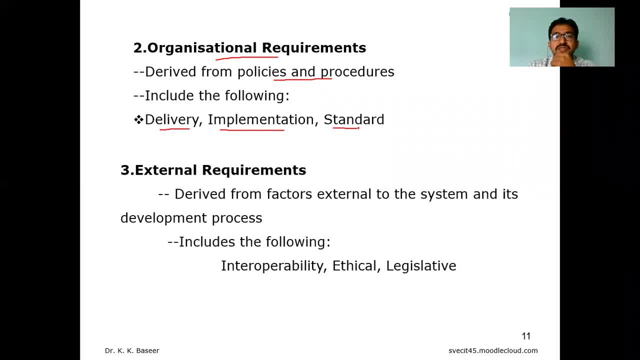 peoples who are living in the society. such type of all standard processes policies will be defined in organizational requirements, like when we have to be go for the delivery of the product, the implementation under which we can be implemented. how could. it will be suitable for that in the society and 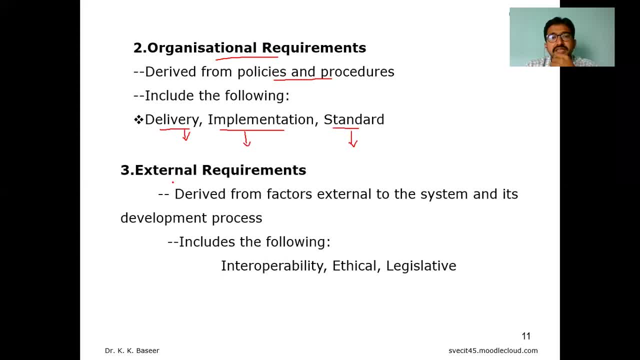 what are the standards? can we follow over? the third one: external requirements. like the name itself talks about, external, external requirements derives with the factors from external to the system, like interoperability. interoperability, ethical legislative interoperability is nothing but when you are going to be adding this, your product, externally to any device, external way. 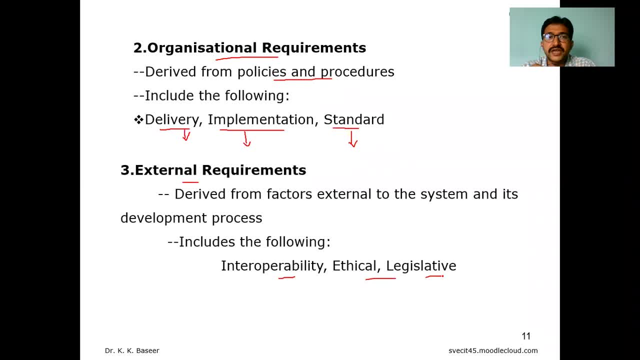 now how good it will be, supports to that existing configuration and to your, the new configuration for your project, whether it is suitable easily for that one, how good it will be, how good the interoperability will be there best. another example: you are having an ATM, for example, the. 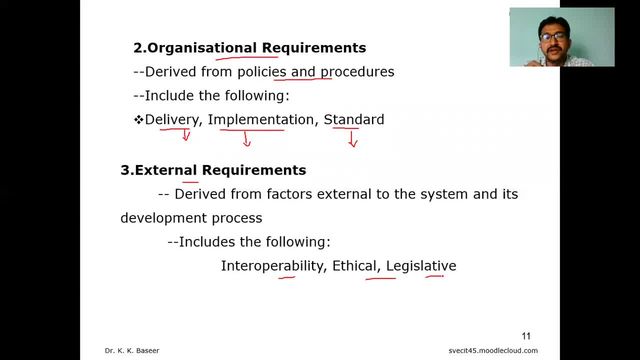 banks having the ATM. they are going to be make some ATMs in different different locations in that particular locations. how good it will be supports whether definitely AC has to be required or not. so that's the first one. the second one is how good it will be, how good the interoperability. 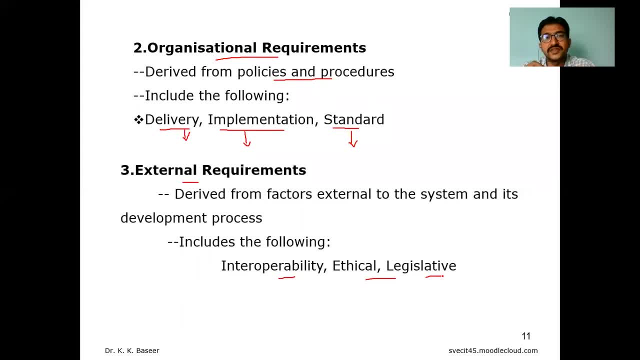 is AC has to be required. the AC, whether it is, supports for that, the maybe more number of transactions will be there. if one machine is there, one AC is enough if it is more than like for deposit machine. another two transactions or another passbook making, printing, all such type of 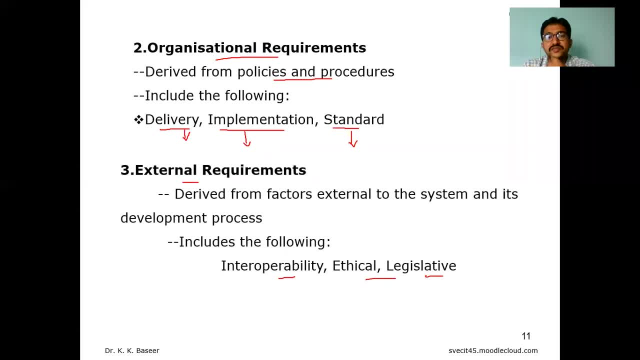 machines, more and more number of machines, how good the different ACs will be, supports, interoperability, deals with. when you are integrating this to the system, that system is the only. your project is the rest of the system. the rest of the things has to be. depends on that. now, ATM is only your part. the 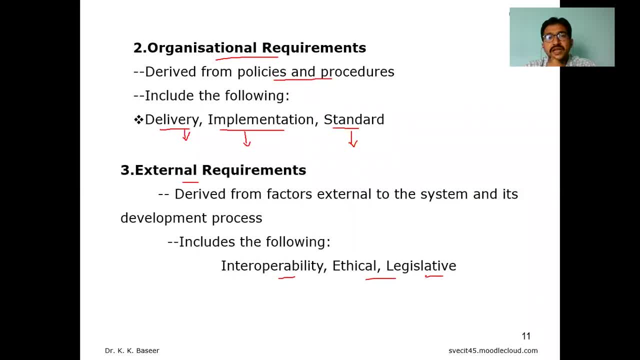 rest of the that other is the power, the environment, the place, the ACs, everything is the other people. when all together, if you don't have any problem, then the services can be fulfilled. if any problem comes with the external party, maybe from the AC or from the environment or from the power, then 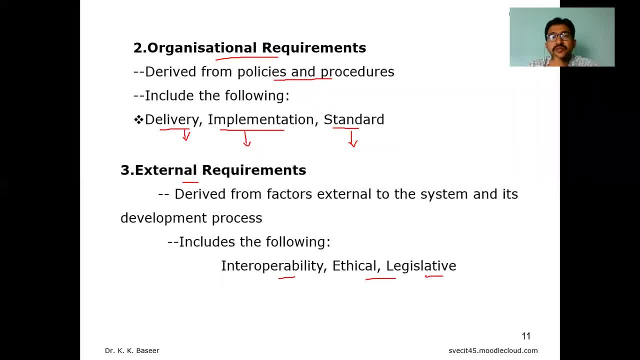 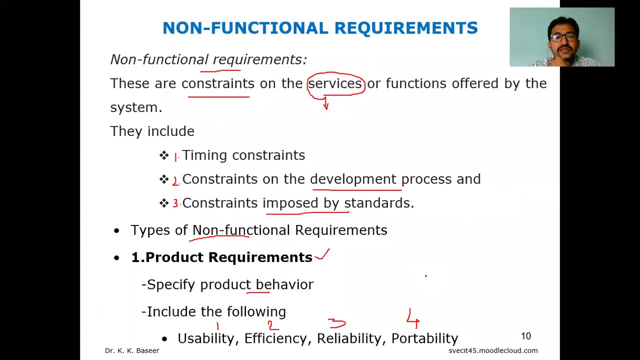 that type of problems will call as interoperability. so it is going to be coming as external. so it is inter means what it's coming as external outside, ethical and legislative. all such type of requirements will comes under external requirements. clear now. these are the three NFS. one is product. 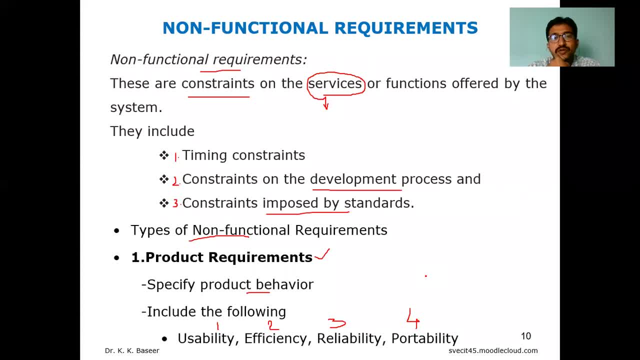 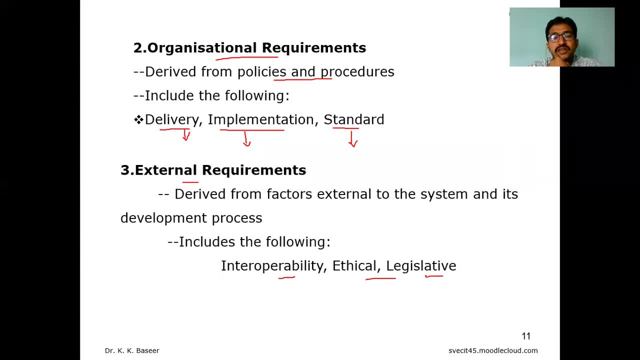 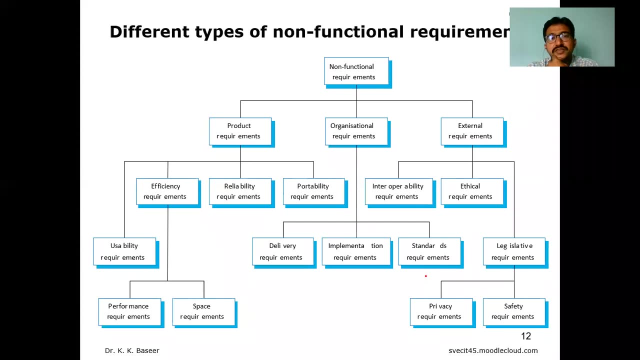 requirements under which we have usability, efficiency, reliability, portability. under the organizational requirement, we have delivery implementation standard. under external requirements, we have interoperability, ethical legislative- if you see overall the figure for nfr- non-functional requirements, as I said you, it is we are going to dividing into. 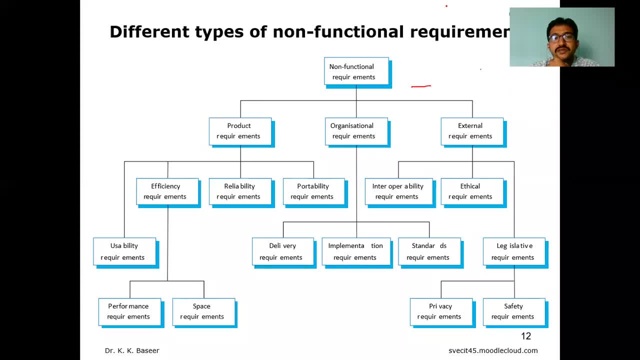 three parts here. we are going to dividing into three parts over here. the first is product, the second one organizational, the third one external. so whatever we are discussed, just all under the product. what are the comes under usability? this is 1.1. next efficiency, 1.2. next reliability, 1.3. next. 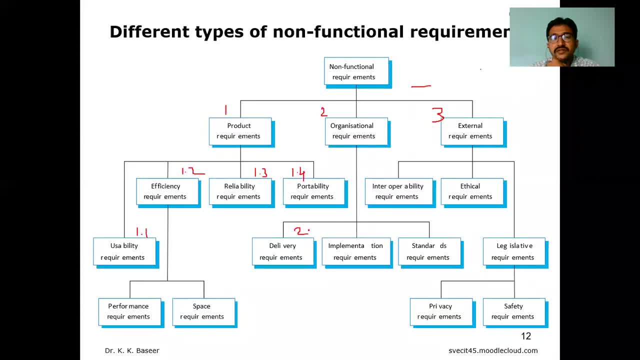 performance and under organizational we have deliverable, that is, delivery, 2.1, implementation, 2.2, standards, 2.3. under external, we have again three, that is, 3.1- interoperability, 3.2- ethical and 3.3- legislative. and if you see, the efficiency can be calculated with the performance 2.1.2.1 and also. 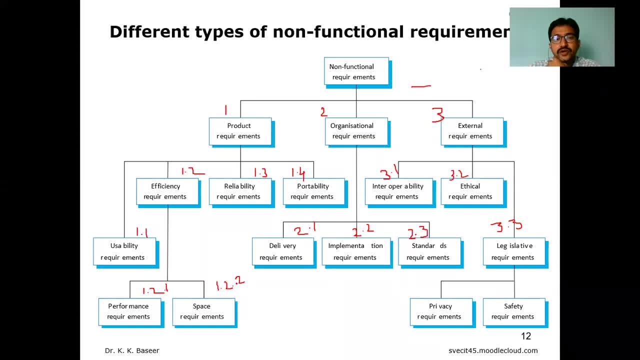 with the help of space 1.2.2. so efficiency not only we can measure directly, we can take the help of performance, like how good it is responding for your request and how fast this service is providing, and how the spaces is going to allocating, how good your program is running, as well as the space. 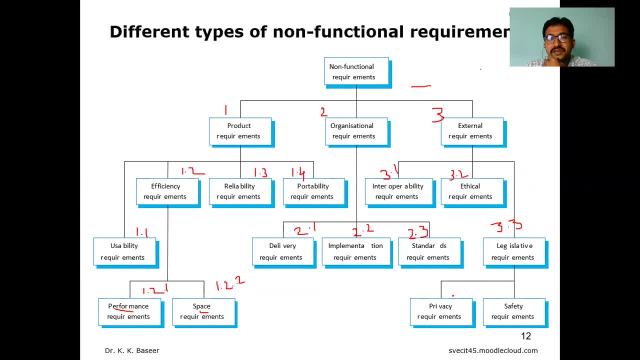 and legislative requirement. again it is deals with the privacy. this is three point three, point one, and three point three, point two. so like this you can draw a overall picture which can be suitable for this one. okay, so whatever we have critically talks about in a graphical representation, it. 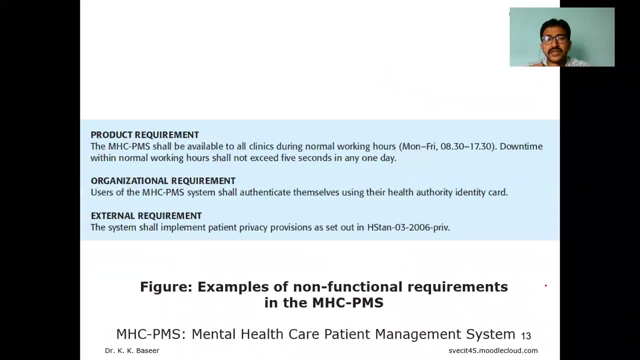 is represented here and if you take one example, the same example of, we have MHC, PMS, that is, mental health care, patient management system. MHC stands for mental health care, the, the patient management system. so we have discussed in a nfr three, that is product. the second one: 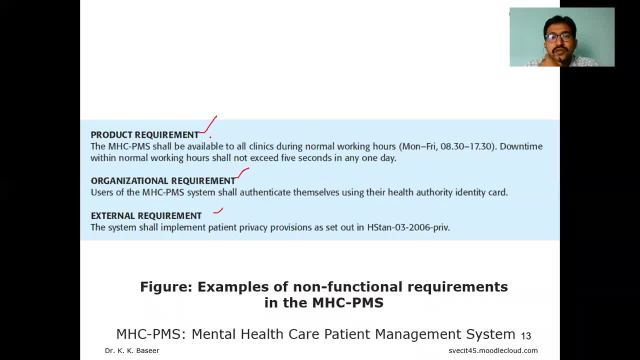 organizational. third one, external. if we talk about the product over here, the product is consisting all the clinics. we are going to be searching for that. so in this one working hours- normally it is monday to friday- 8, 30 to 5, 30 normally. now the product requirement is the downtime with normal. 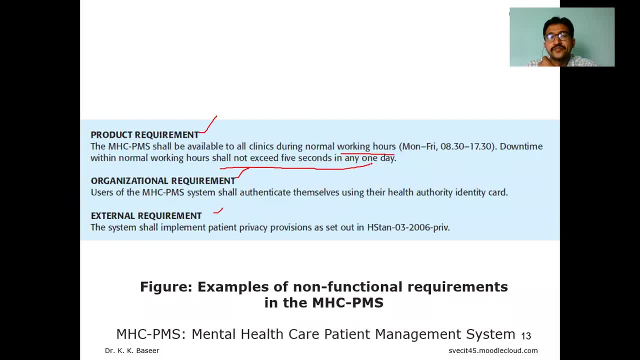 working hours shall not be exceed five seconds in any every day downtime. in the sense if any problem appears in in the working days monday to friday, within five seconds, within five seconds, the problem has to be rectified. the downtime. it should not be exceeded more than five seconds. 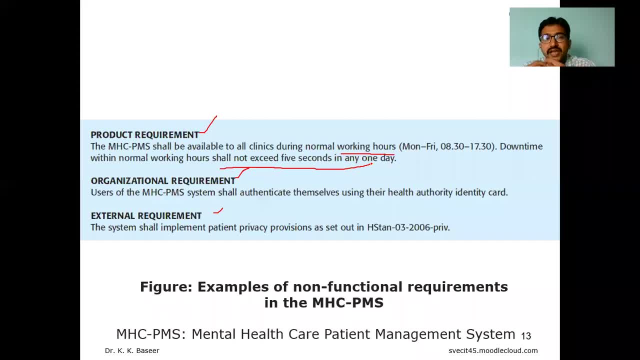 such type of requirements. we are going to talking in product. if you see, organizational they are defining using there some health authority identity card like every. uh, we have our registry card, you in the same way here for the authenticator, peoples who are eligible for that or this records. 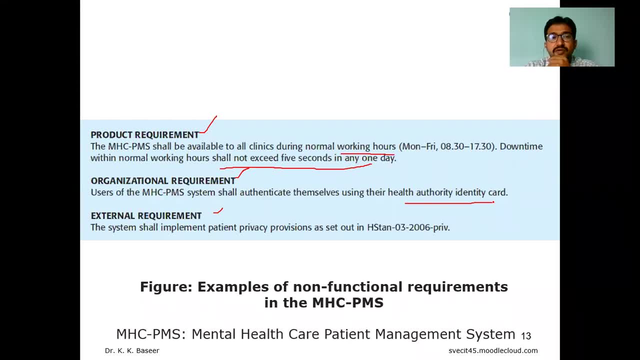 they have, like health authority identity card. such type of requirements comes under organizational requirement. external requirement will deals with the privacy provisions. privacy positions is set out in the privacy positions is nothing but like all the diseases should not be revealed to a very party, because some diseases can be hide, some diseases can be revealed. so 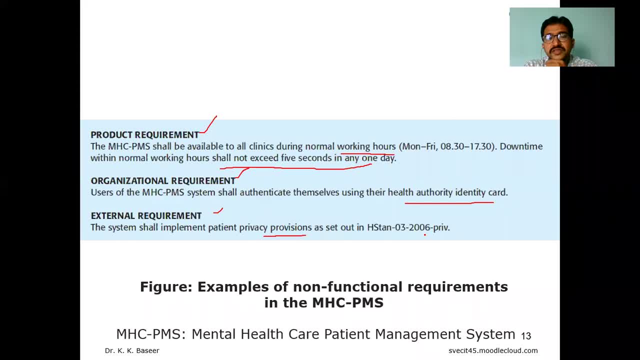 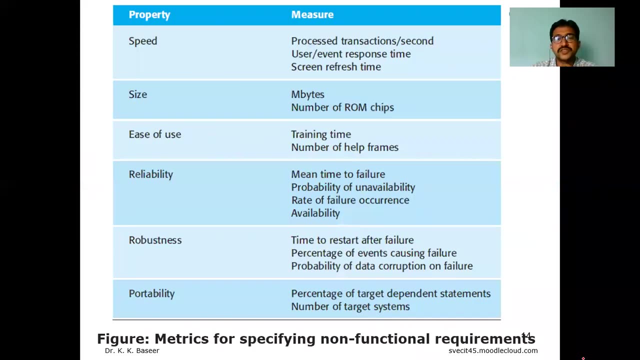 because of some diseases which can't be revealed, so that the peoples can be seen a different way. so we have some for the maintenance, some privacy for the patients. such type of requirements will comes under as an example here: external requirements, right, so if you talk about the metrics which are going to using for nfr, non-functional requirement now already. 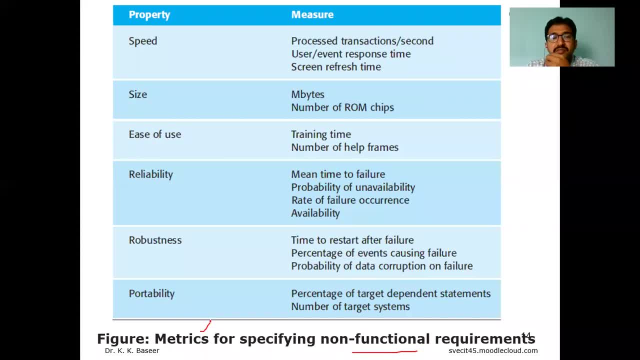 had defined you in the week, to a metric means. metric means what a measurement? maybe with respect to quantitative, with respect to quantitative, if you measure, then it's completely different from the measurement with respect to quantitative. with respect to quantitative, if you measure, then it's game from the tablet matrix. so 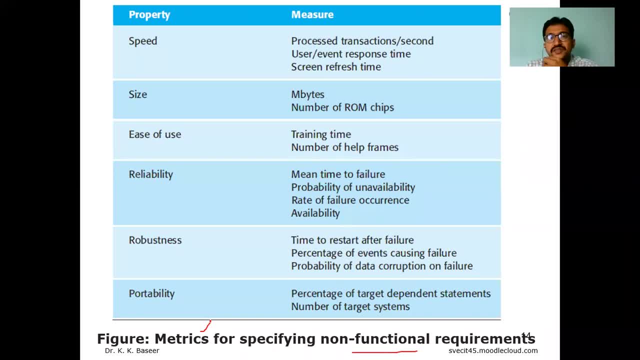 the matrix, for again we'll talk about in the fourth in it two types of methods that have product metrics process, but it has part of you how, in effect, functional governments are going to be measuring, making some nexus plus metric custom. and the third is a few reliability over than forty. now all the step of metrics. 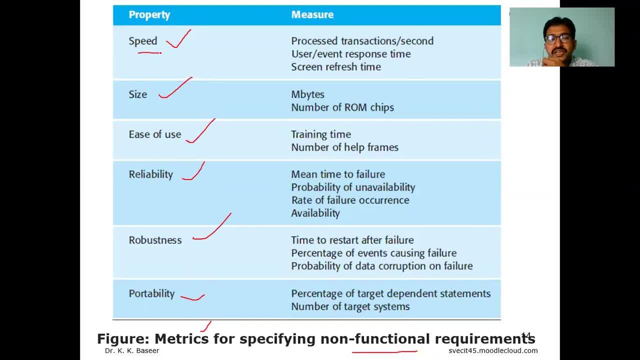 you are going to be measuring, though I now how you are going to measuring a particular speed of a particular project, say, for example, mhc, pms- the same system or same project. how you are going to be calculating the metric. here is speed. now how you are measuring processor transactions, or per second. this is second per user or per second? 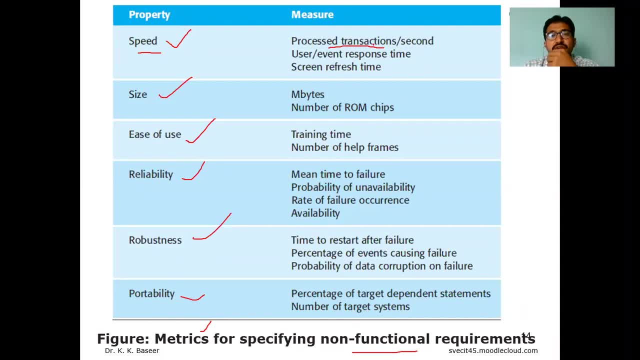 this is a we are performing some transactions. for example, if you are providing a service, how per second, how many number of transactions, how many number of services you are providing, or user versus event response time, when user is asking some request, how the response is coming. that we based on that also, we can based on that measure also, we can calculate the metric called. 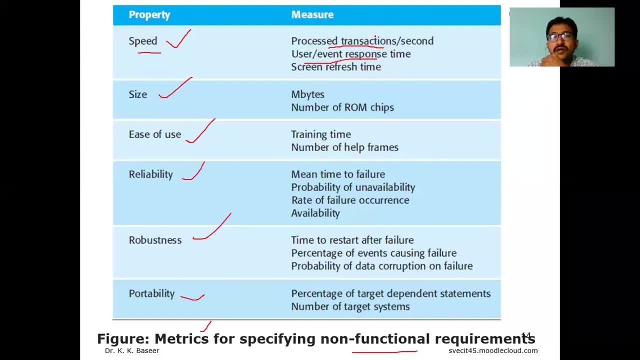 as speed screen refresh when i click fi or right click refresh. now how much of time, within how much of time, it is going to be giving the new page, refreshing that page? that also here comes under the speed. so this is the speed that we are going to be giving the new page. that also here comes under the speed. so 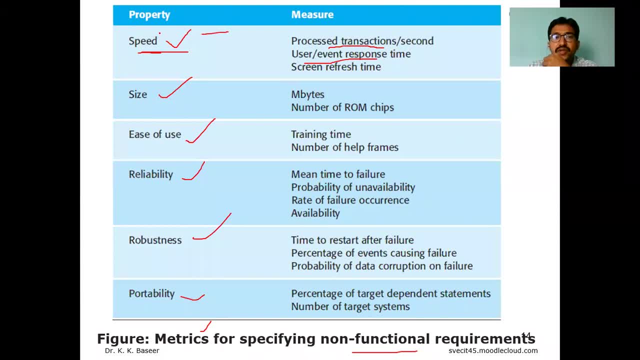 these are the three different uh my measures where we can. uh deals with speed metric in same fashion. size size can be measured in mb, that is, megabytes, or number of the chips of read-only memory rom- wrong chips. it is going to insert it. based on that we can define the size. ease of use. 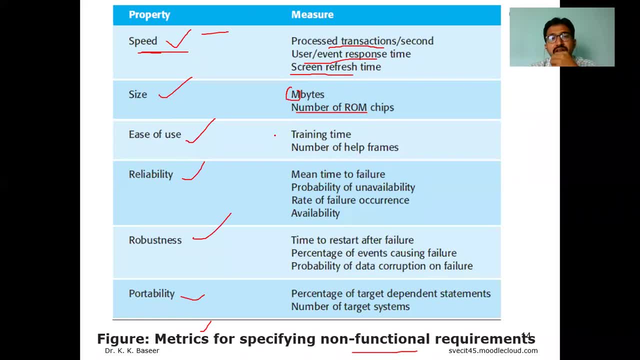 means how good easily one can learn how to use your product. most of the apps. initially you don't know, initially whatsapp. also you don't know how to use it. but whether you have taken any training further for learning of whatsapp, whether you have taken any training for how to use the phone. 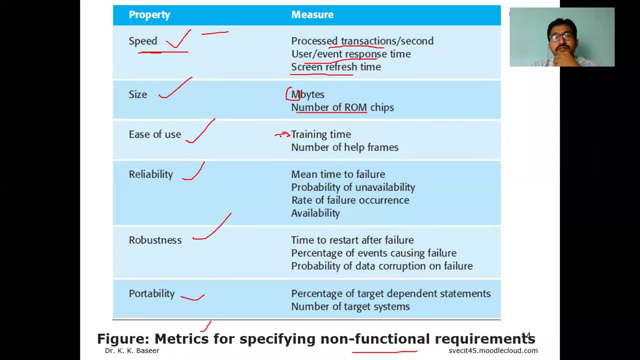 based on seeing some options, by based on learning from friends, you can learn some apps, some systems, some projects, whether it is required any training time, whether it requires any number of help frames. based on these two measurements, we can calculate use of use metric. coming to the next metric, 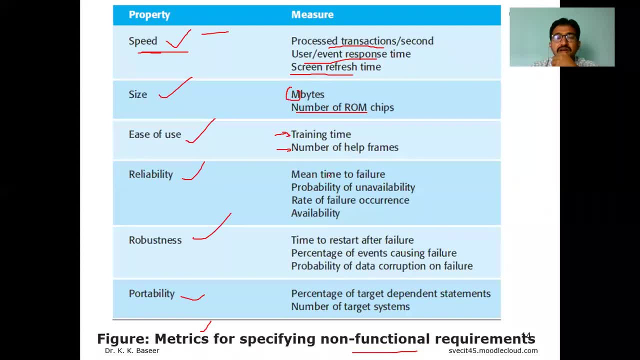 reliability, mtr that is empty. the mean time to failure, the mean time mtf. you can also use mean time to failure. mean time to failure means in how much of time, how much of time it will be get whenever a system fails, it is recovering, it is rectifying order. any fault occurs. how much of time? 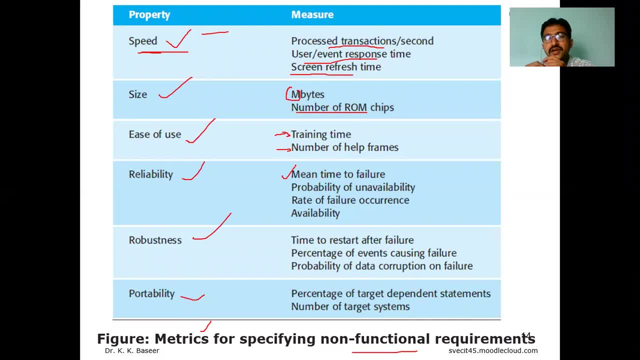 it is taking to tolerate that and taking to recover, and probability of the unavailability, how much of time it is not available. so how it is going to be calculated over there. rate of failure occurrence so frequently for every year the repairs, or every year the system is failing, or 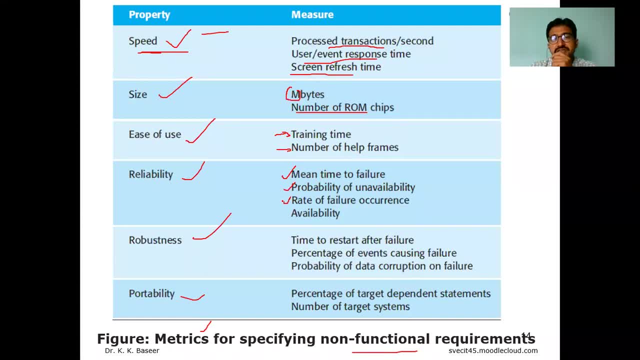 for every month- is failing. what is the rate of frequency occurrences- every month or every week, or every year, how it is failing and how much of time it is going to be available? this system, based on these four measures, we can calculate a metric called as reliability. and, coming to the 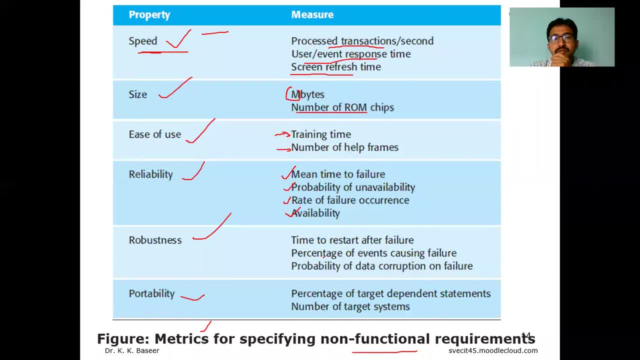 name itself talks about: robust means strong, so time to restart after failure. how much it is taking your system to restart further, percentage of events causing failures. probability of data corruption on failure. so all these three measurements will be used to calculate the robustness factor, right. and the next is portable- the name itself, portability for any system. 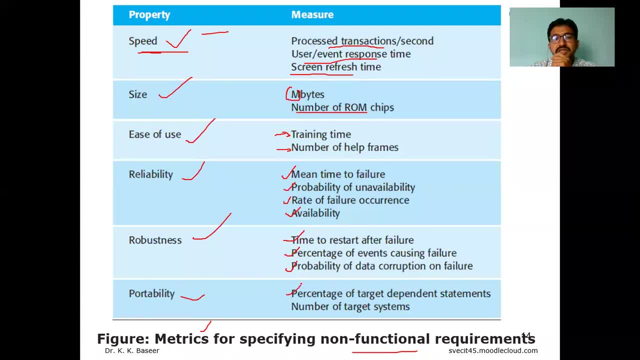 target dependent system, the number of target systems, percentage of target dependent system. only for suitable applications it is going to be. for what is the percentage number of target system for any number of systems it is going to be making portable. it is going to easily adaptable further. all such type of things will be talks about in the matrix of nfr. so speed, size, ease of use. 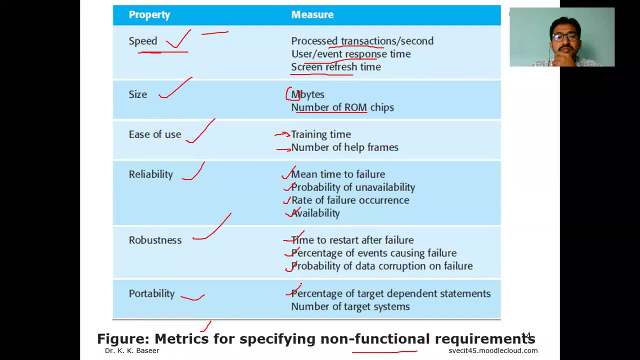 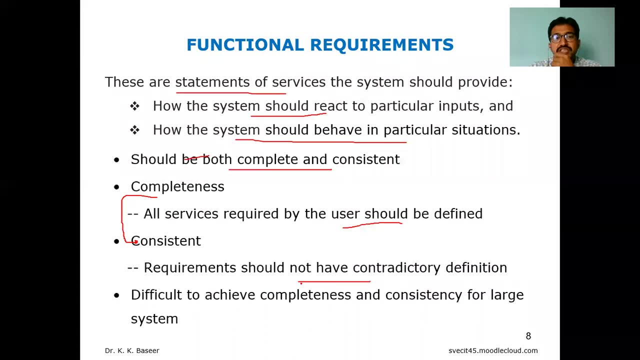 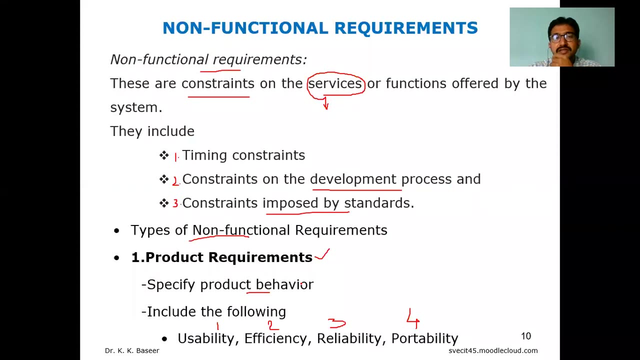 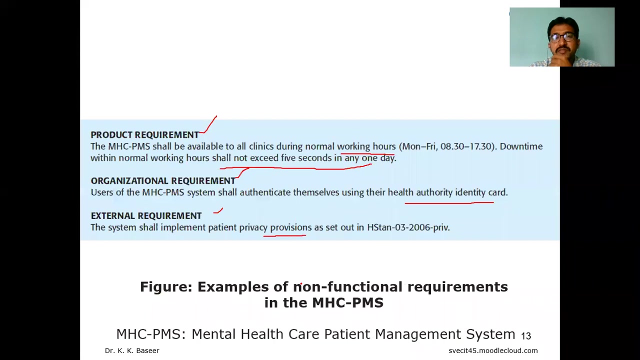 reliability, robustness, portability- all these are the metrics and respective measurements over there. so just now we have discussed about the functional requirements- how it will be workouts with an example, and also non-functional requirements and again the types of non-functional requirements, which is some graphical representation, also one example for nfr, with the help of the mhc pms system and the metrics which 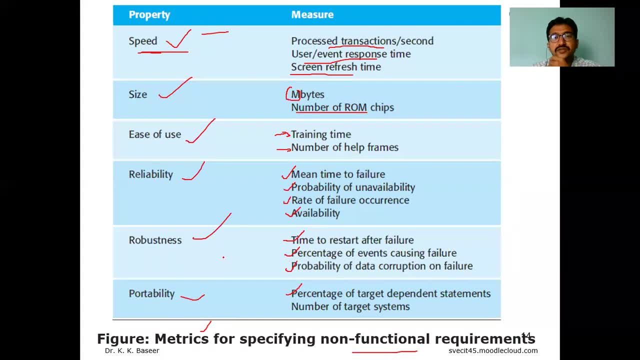 are going to using for nfr. so that's about functional requirements and non-functional requirements.